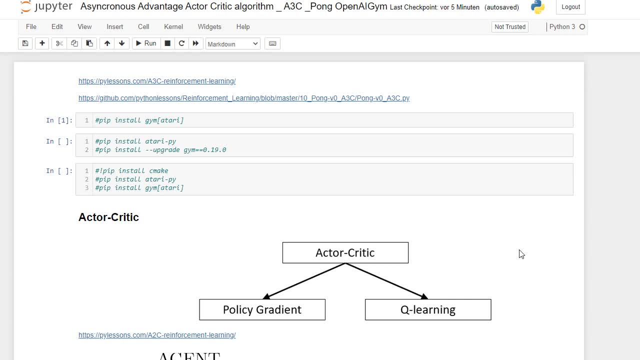 Hello and welcome. Today we'll talk about asynchronous advantage actor-critic algorithm. I will show this example with Pong game and I'm using for this OpenAI gym. So welcome to this lecture. My name is Haris and let's get started. 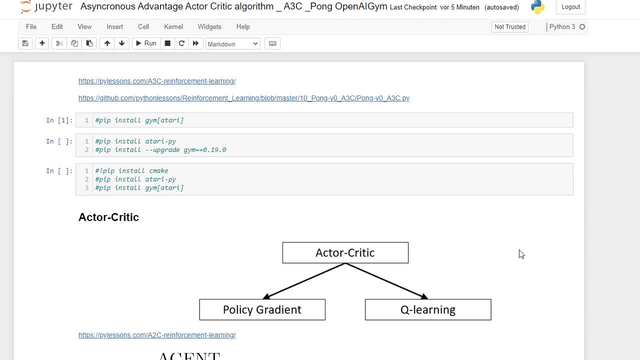 So this is a Christmas edition actually. So if you like it, if you like the content and you want to see more of these topics, please, I would be really happy to receive a nice gift this year, So you can hit the subscribe button or leave a like comment there. I'll be really happy about it. 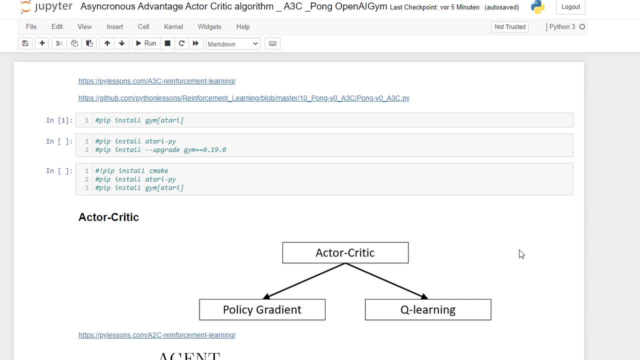 So many guys of you were writing me the mails or were discussing about the next topic, So I received a lot of attention for the A3C. So I wanted to discuss today and to show you how you can implement The A3C actor-critic with Python and how you can, and I will also explain what is it about, about this advanced algorithm. 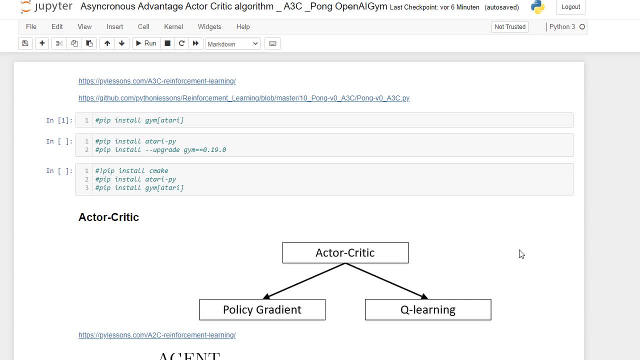 was introduced by DeepMind and I want to talk about it, how you can use it to understand a little bit the topic itself and how you can use the code by yourself. You can find my code. It's actually in GitHub, So if you like this part, just grab the code and try it by yourself. 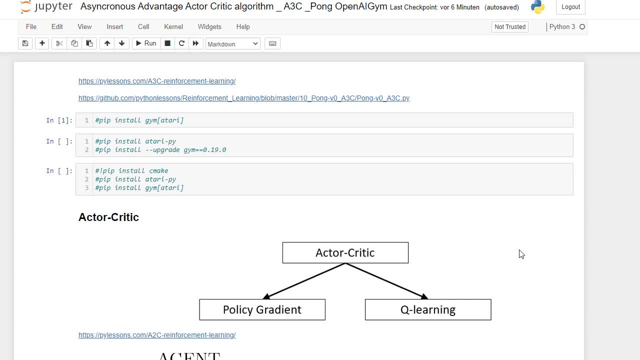 And I'm really happy if you can, you know, send me some response of this and how you like the code, if you can handle with this code and so on. And yeah, we can talk about it and hopefully this code will help you. 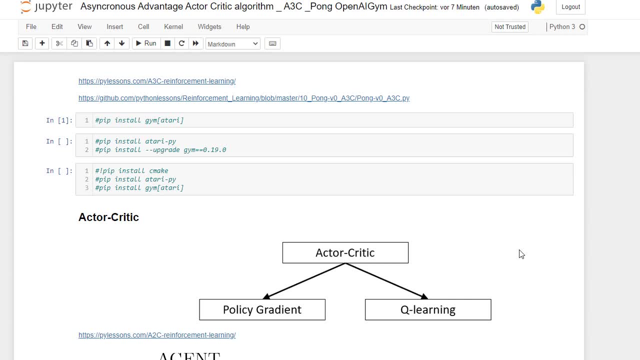 To get better into this topic, to use it maybe on on on on your project or at home at your private project. And yeah, this is my goal: to just Yeah, to just send you or to yeah, to make it possible for you. 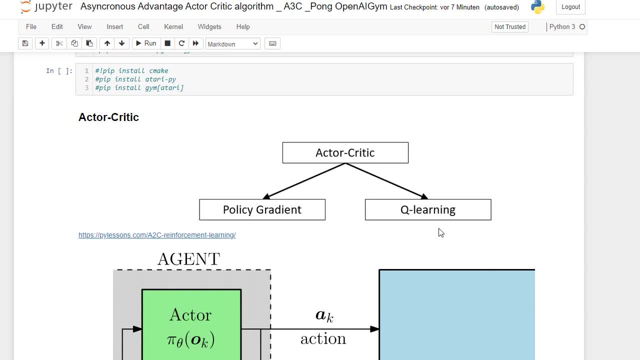 So, to just wrap up what we're talking about- because the first, very first, lectures about reinforcement Learning, we're talking about actor critic- why this is such a nice and really powerful approach which you can use in reinforcement learning, especially in a continuous environment. 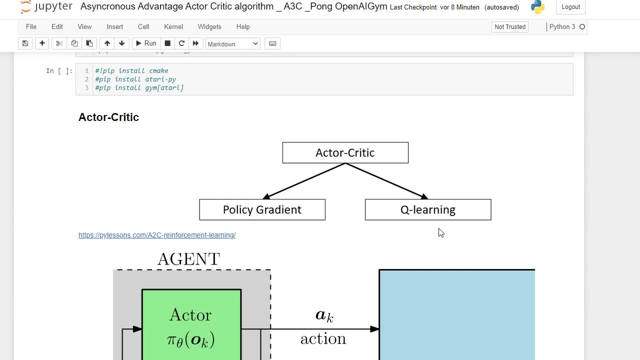 So to just wrap up what we're talking about last lessons, let's get started with actor critic. So, as you can see here, the actor critic is using actually Once if you see the two branches, you can see the Q learning itself. 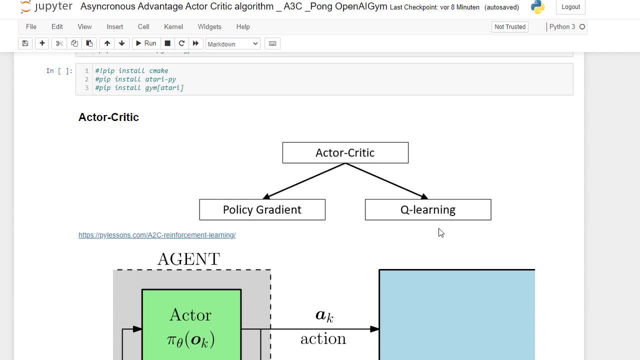 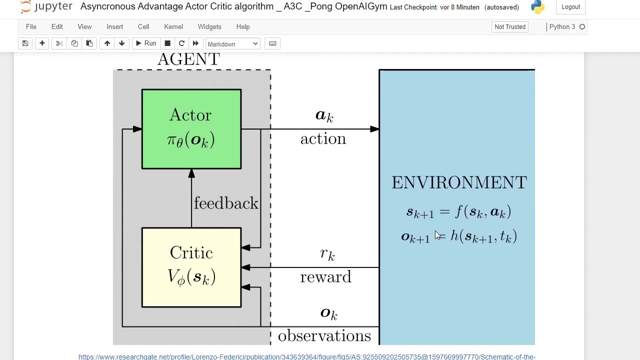 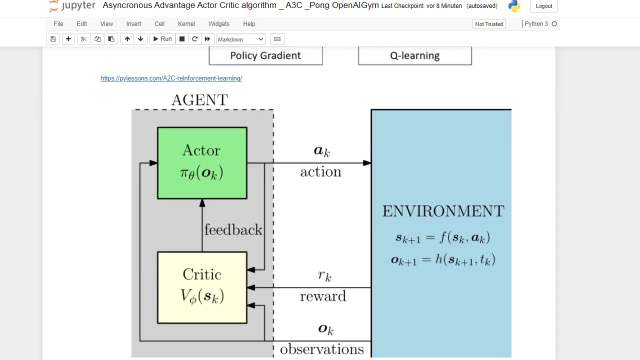 And you can. he's also as well using the policy gradient, So both of these worlds are getting together. That's why this is such a powerful one, combined in all in one solution, And This looks like following that, you can, you have to. on the very left, you can see the agent. 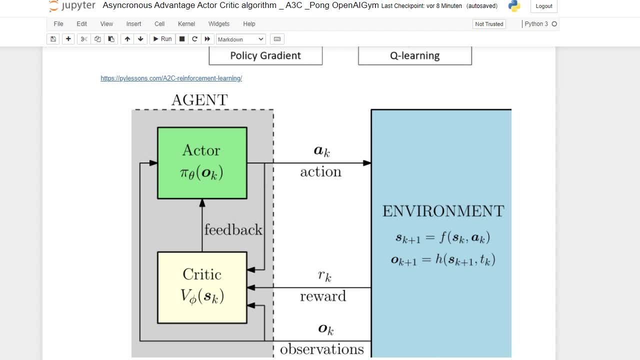 Where you have The agent is actually represented by the actor and the critic. So the actor is Calculating some action, Then receiving a reward and observation from the environment itself, And the critic is actually Receive or giving the actor some feedback on the. 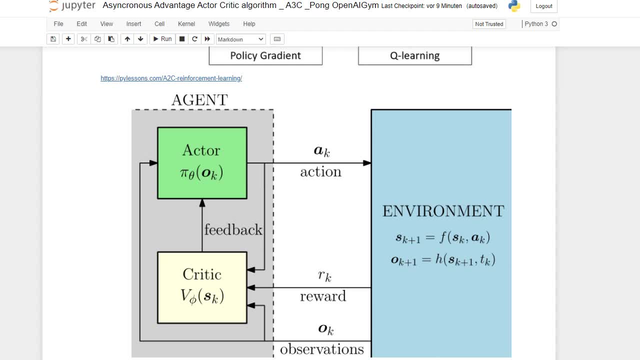 Calculated action that he was taking right. So this is something that you can imagine with with guns, generative advertising networks, Where we have also a generator, and then you have discriminator. This is something as well like this: So you have an actor who is, you know, calculating through the DQN. 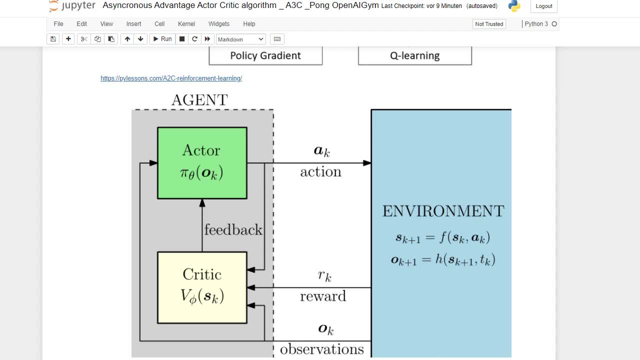 He's calculating the action based on the state, And then he's receiving a reward. And then he's receiving some feedback from the critic Like hey, guy, you've done a really nice job. Or hey, this action was not properly done. 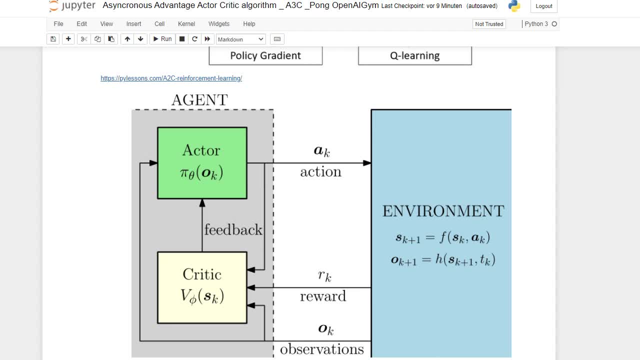 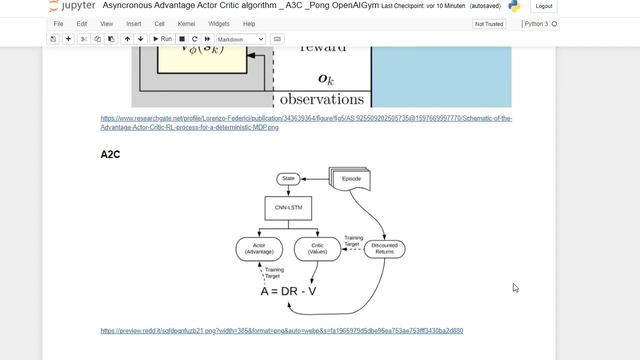 Maybe you can do it next time better. So he's receiving some good or some bad feedback. Of course, each action, Who is where he's calculating and taking on the environment. This is pretty, pretty good approach. So The A to C. 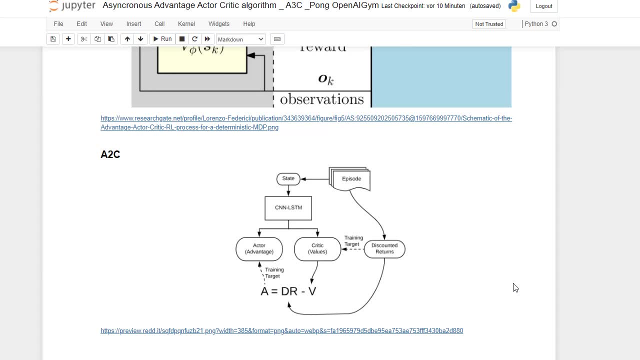 So the advantage Actor, critic is actually using or calculating as the word saying the advantage Right. So you have the actor and the critic again Which are contributing each other And each Episode the Actor is actually receiving a discount return And 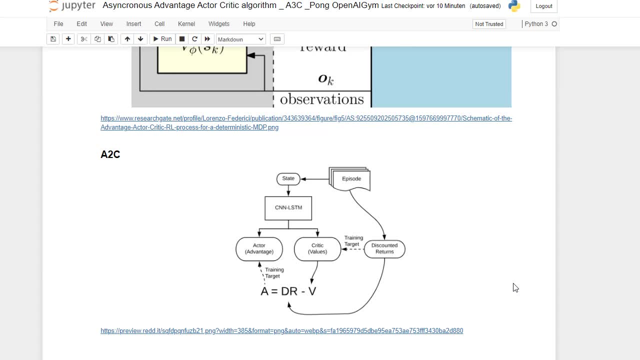 The critic itself is calculating the value. So on the left hand you have the actor who is calculating the advantage, And the critic the value itself. And this got Subtracted To. You know, the aim is to just Calculating the advantage itself. 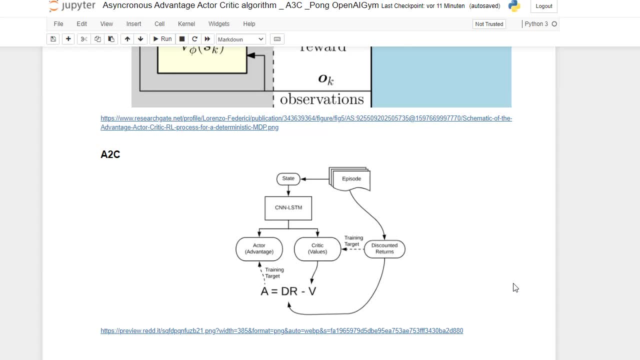 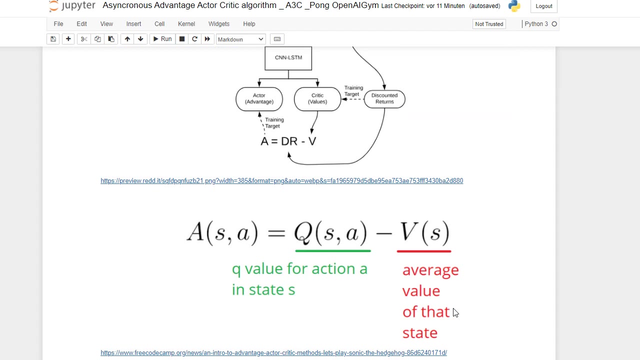 And to minimize the loss. So to make the network even Faster In respect, to Receive a higher reward in a faster time And to Have Lower loss. So To just improve the network. Right To just see the calculation. 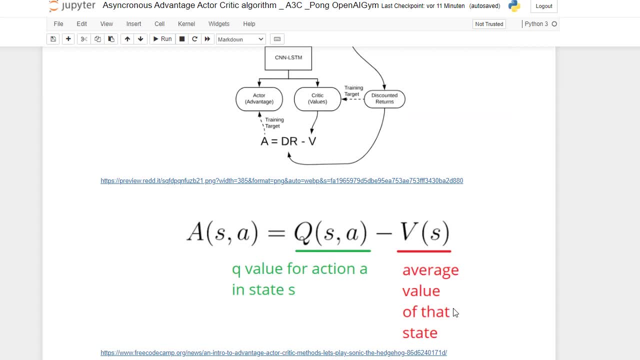 You can see here The Q value For action A in the state S And subtracted by the Average value Of the state itself. This is the advantage. This is a basic Calculation with Which we were Setting up in the 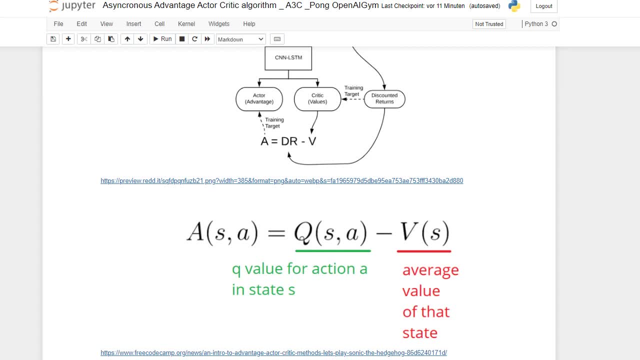 Code. You can also find it. I will show it Afterwards In the next Video, In the next Video, In the next Video, Afterwards In the path Code On which Position We were using This. 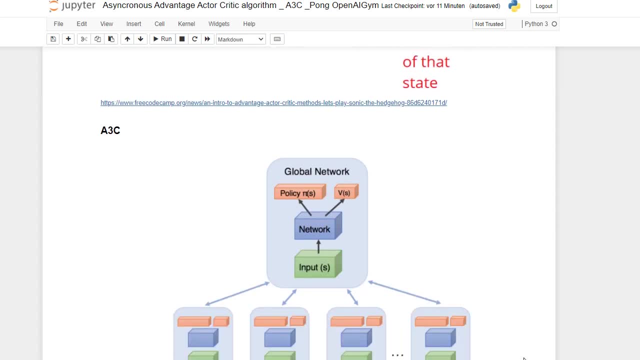 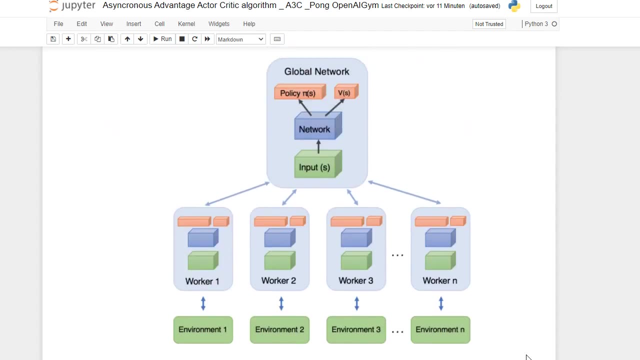 Very important Equation And This Equation Is Going To be used At A3C Model Again, But Here We have Other State Of The Art Model. This Is: 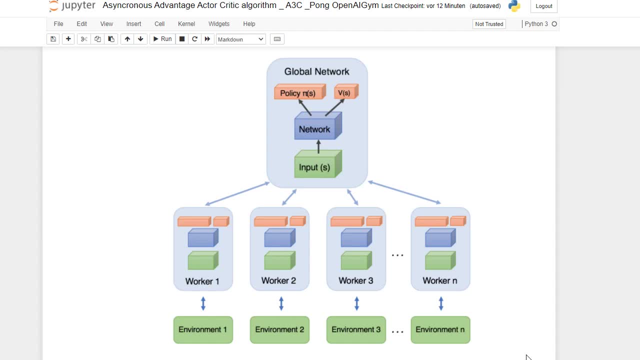 A3C. The Table That Is Going to To One State Of Calculation In The Model A3C Model. Next In, You Have To Use A3C. 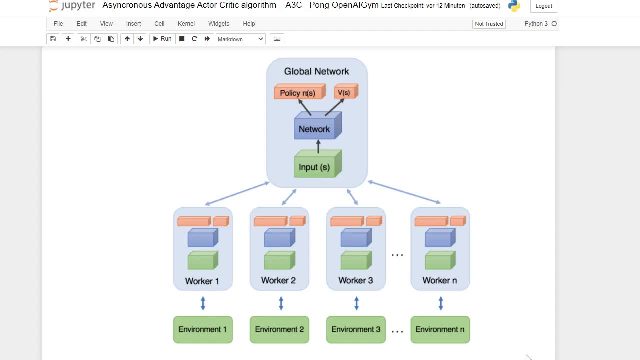 On The, They Can Save The, the blue, and then you are receiving the input itself as the environment and in this phase it's not discrete, it's a continuous environment and, as the name itself is mentioning so, it's a asynchronous network, which means you can imagine this like this: 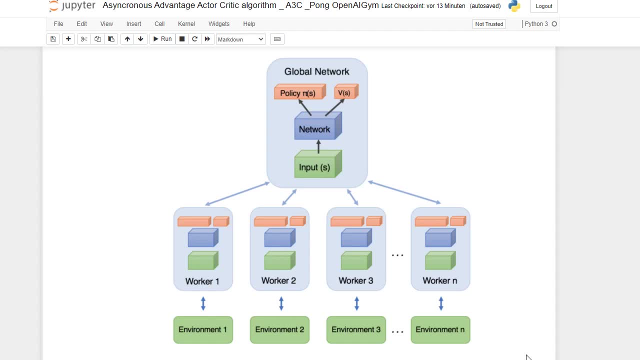 you have here four workers or four agents who are contributing to the global network and they are as in current right, so of course they're working in parallel. it's like parallel treats, but they are. you can imagine that one agent is faster going through the game, the other needs a little bit. 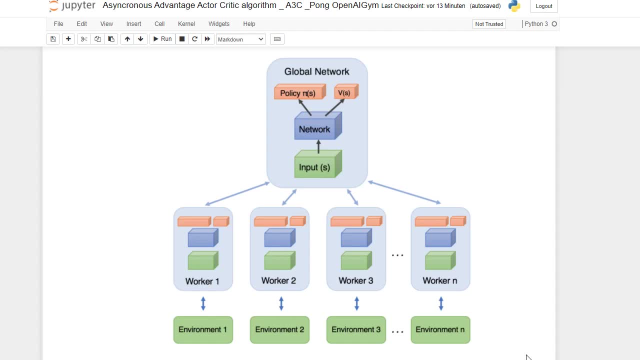 more time. so all of them are contributing to each other at their at output and the reply or the experience from each agent through the environment it's get getting collected at output gate and it's going to be averaged and with this experience the global network can contribute. and can you know um have the best of all of them. 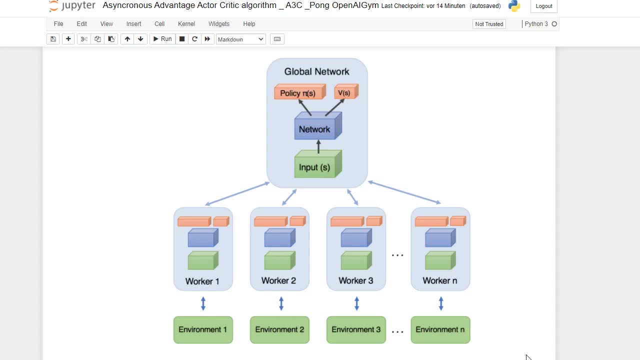 and that's why this global network is so powerful, according to the other actor critic networks. and yeah, this is something that you can imagine, like when you have decision trees and you have one decision trees in machine learning and if you're using a random forest, it has several. 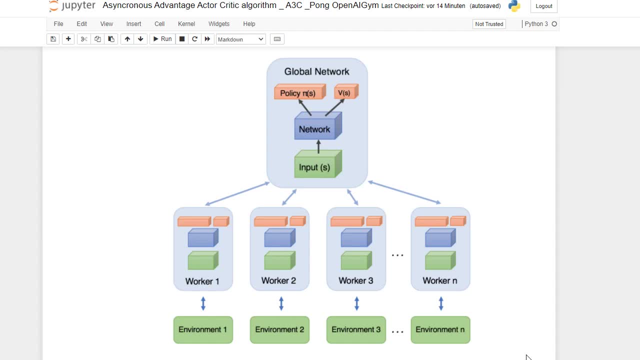 decision trees in parallel. we're going to be um used to be summed up, and then you have a really good contribution, you have a really good result gathered from all of them at output gate and then you have a really good contributed network here. so then we can start with the code itself. 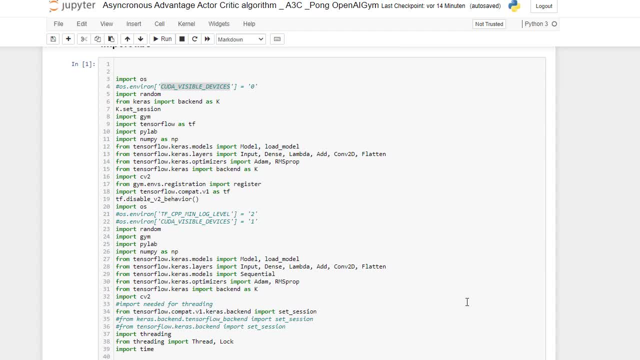 so, first of all, i'm going to import all the libraries that you need here. in my case, of course, you can use google, collab or something like this. if you don't have a gpu, like me, i'm using collab to just, you know, calculate the model. you can, if you have a. 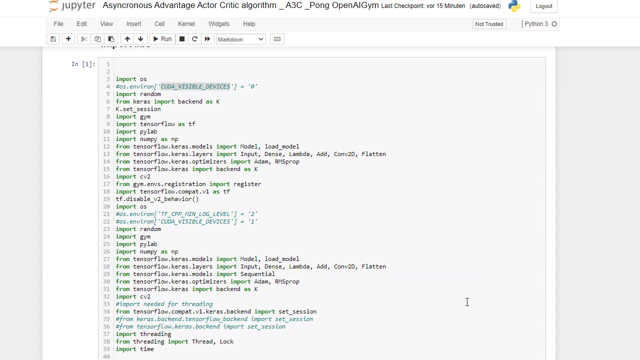 gpu at your computer- nice for you, i don't have. so um, then you can calculate the model and train the model even faster. it took for me several hours to just train this pong environment and the agent itself. so um, and then you can set up cuter visible devices to warn or two, something like this: 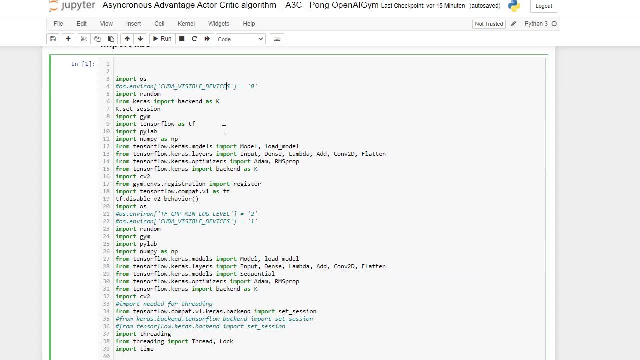 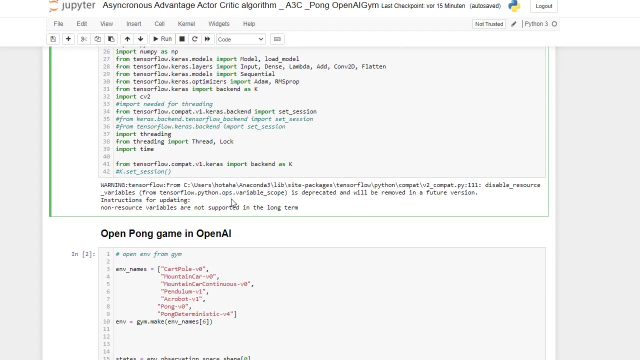 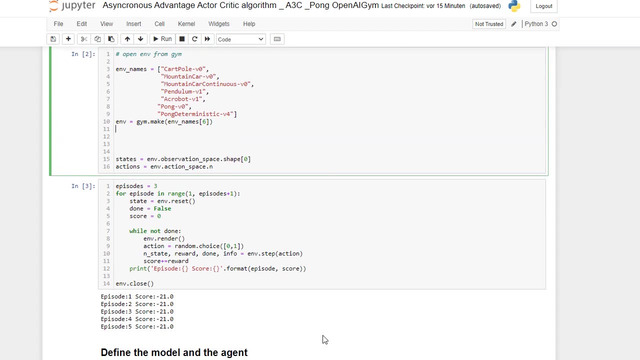 if you have gpu right. so, um, i'm using mostly um tensorfall and kerrox to just train the model. So first of all, I'm opening the Pong game in OpenAI and it looks like this: So this is the non-trained agent who is playing against the other guy. So I'm 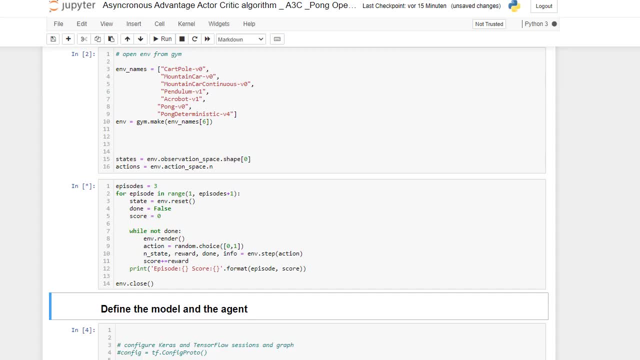 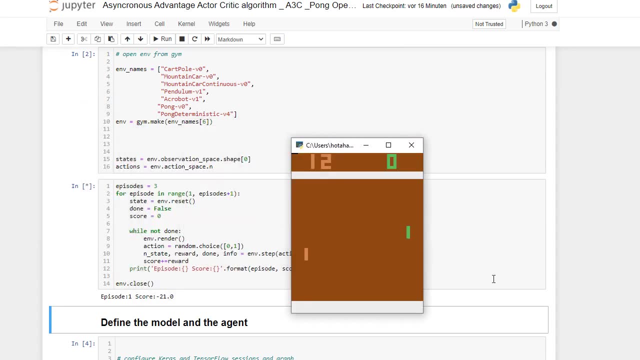 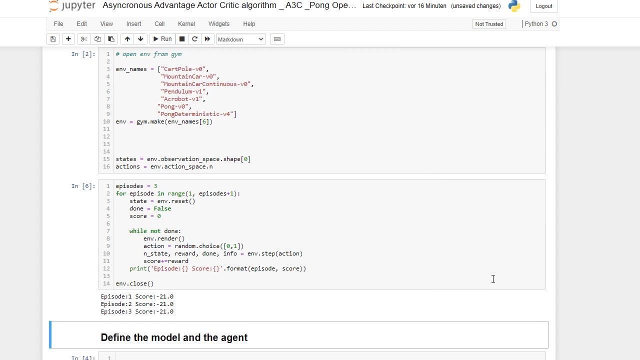 just starting the game to just show you how it looks like. So you can see that he's basically almost doing nothing and he's really bad. You can see that his score is minus 21 and he's hits no points right. That's why it's minus 21.. So the goal of the game is to just receive. 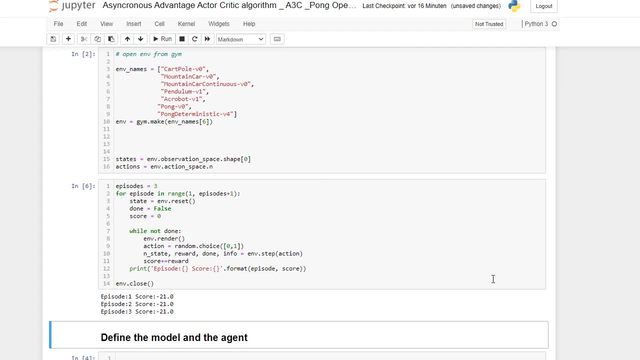 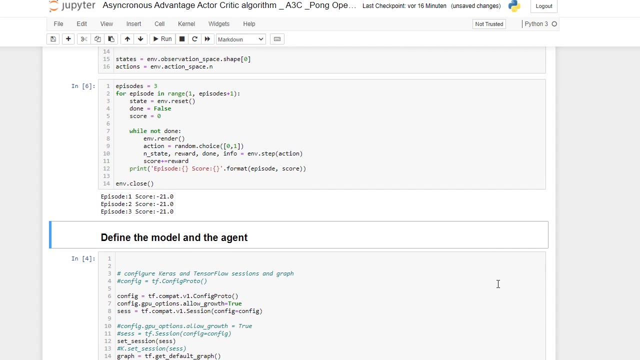 21 as a reward or as a score to win the other agent. So this is the score or this is the aim of the game: to just have more than 20 score to finish the game. So now we are going to train the model, to set up the model and train the agent, And that's why. 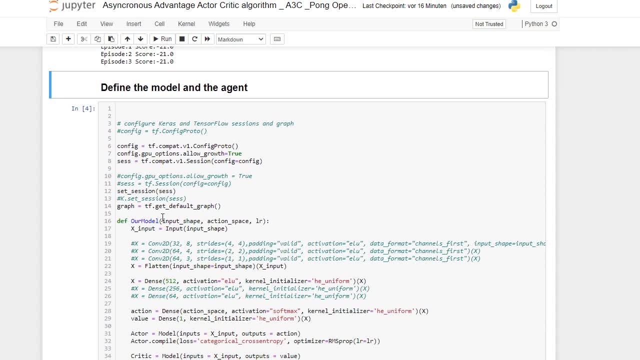 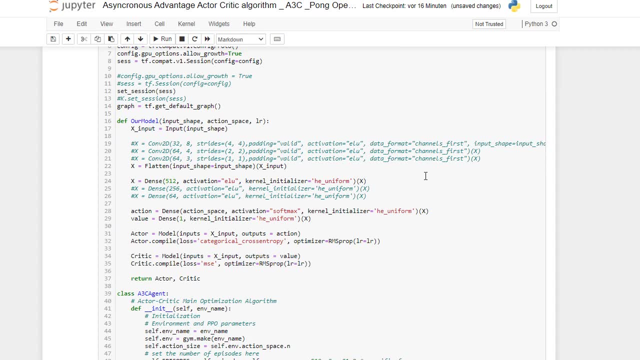 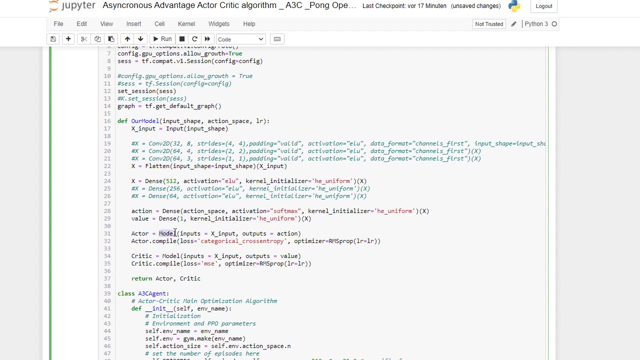 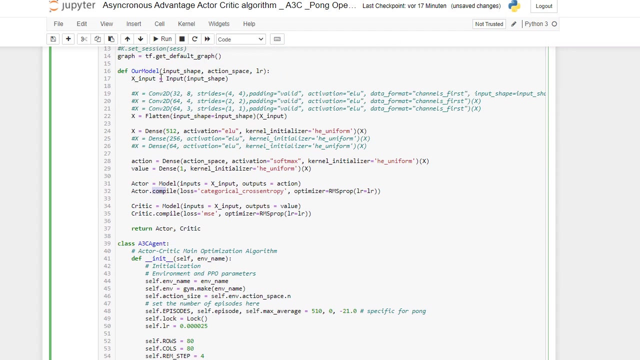 we are getting started here At our model method. I'm setting up the dance layers and so on, And here you can see the actor and the critic itself and how I set up the model. Then they're going to return the actor and the critic itself for the other methods to be used. And here I'm starting. 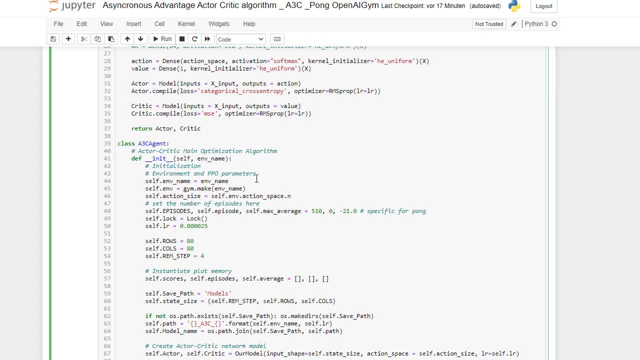 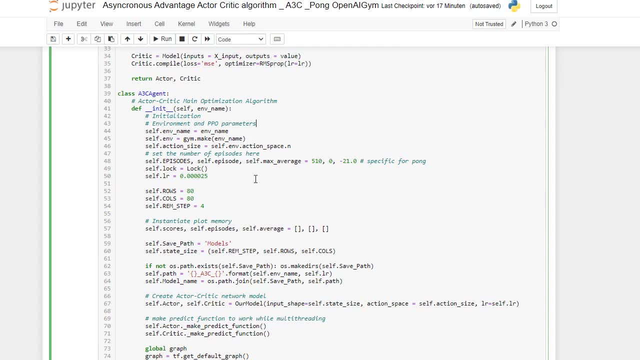 the A3C agent to set up and to basically configuring the parameters itself. Here you can, for instance, set the number of episodes to be more than 10. You can also set it a little bit to 1000 or 2000. 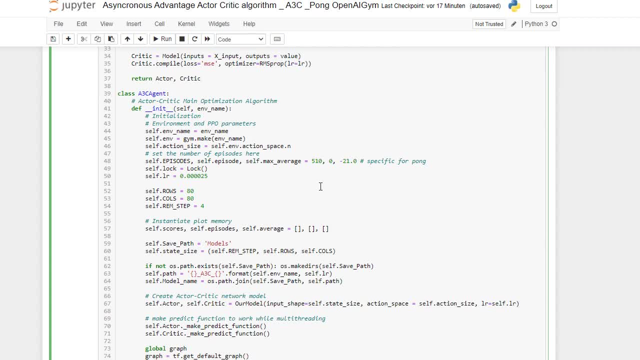 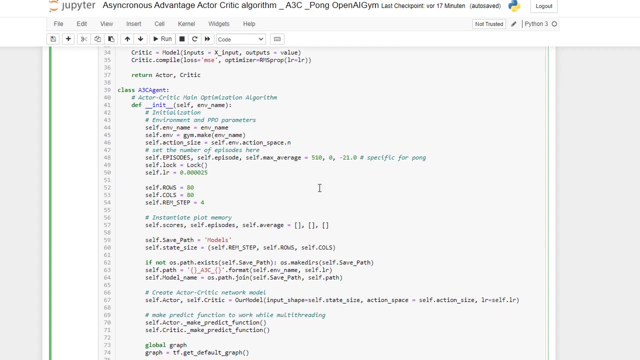 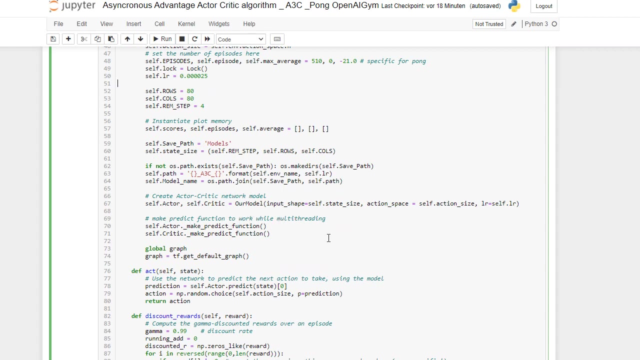 to even improve your agent yourself by training it. For me it took like three or four hours, so maybe at your case it will be faster. Yeah, Then I'm making prediction function to work while multitreating, And you can see that actor and critic, you can basically set the control. 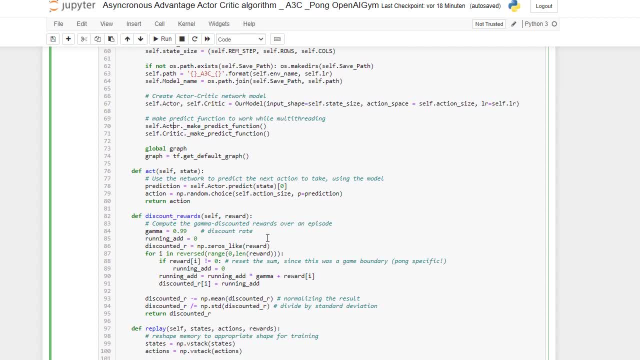 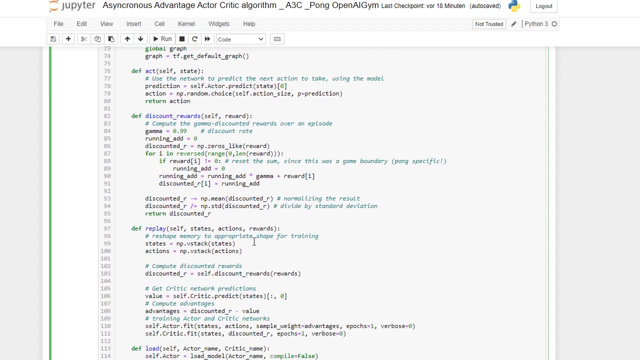 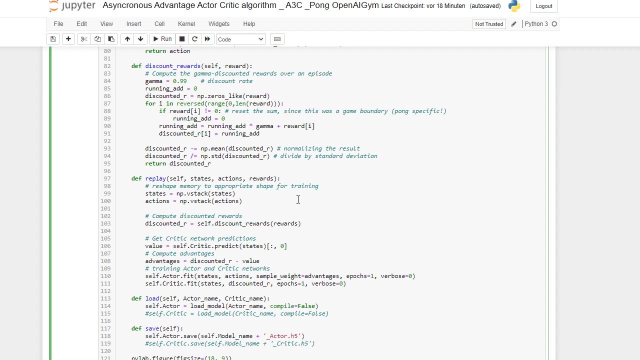 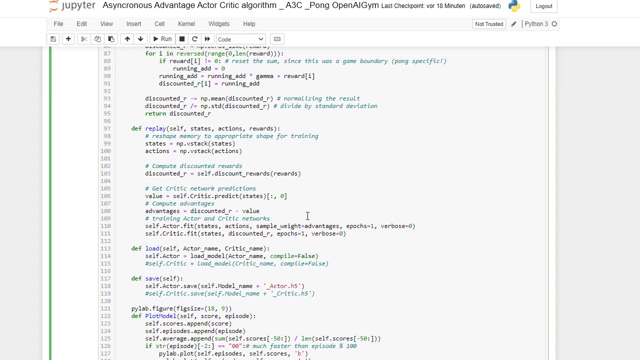 predict the outcome here. Then we have the discount reward that's going to be calculated here. Then we are setting up the memory itself, the reply memory, to appropriate shape for training. Then we have the action and states. Then we are computing the discount reward here. Then afterwards we are computing the. 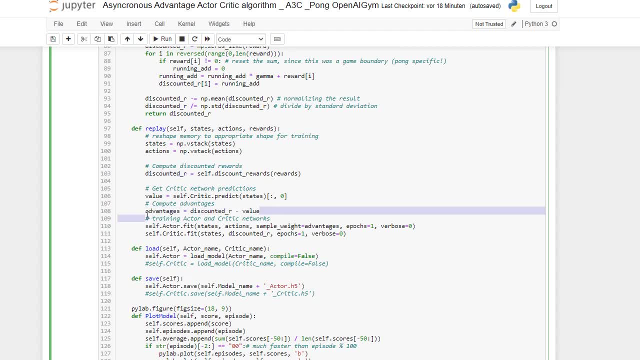 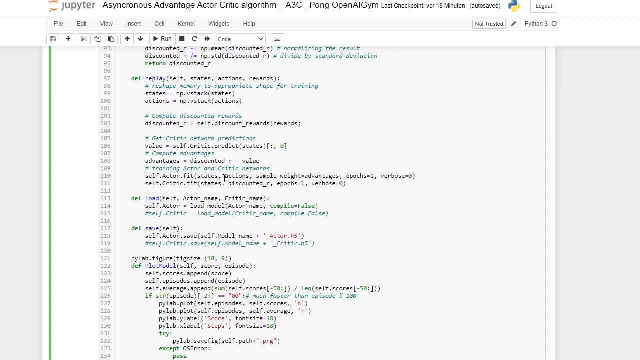 advantage. This is, as you saw, in the formula itself, which I mentioned before. So this is the advantage that is going to be calculated at the discount rate minus the value to be used here in training of actor and critic network. This means that we are going to use the training of actor and critic network. This 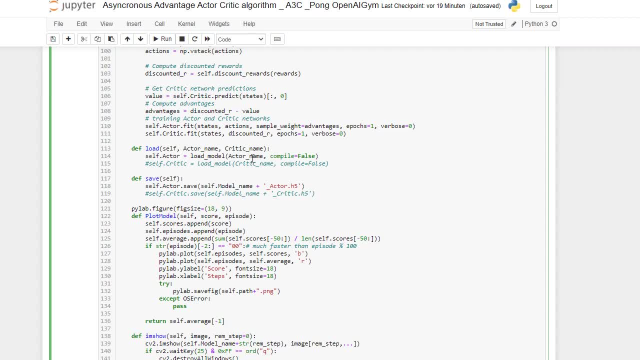 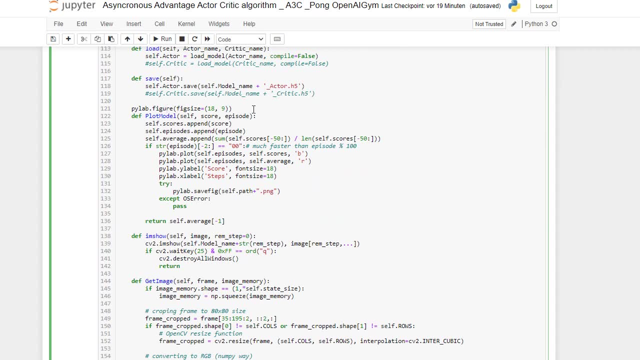 means that we are going to use the training of actor and critic network. This method you can use for loading the model after saving it. After the training you can save it, use it again. The plot method here can be used to just plot. 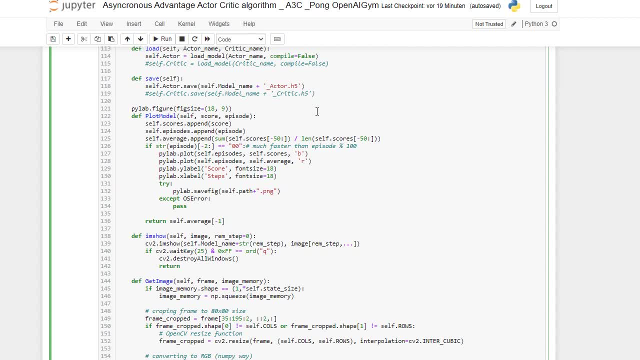 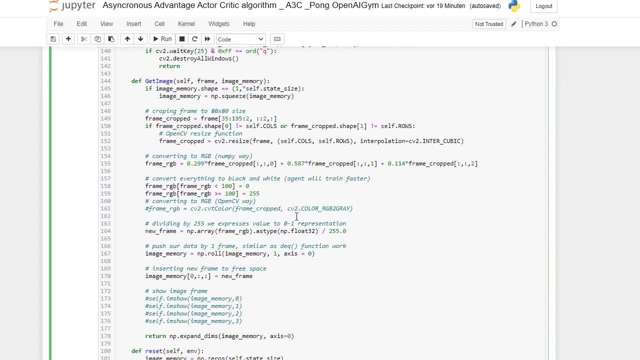 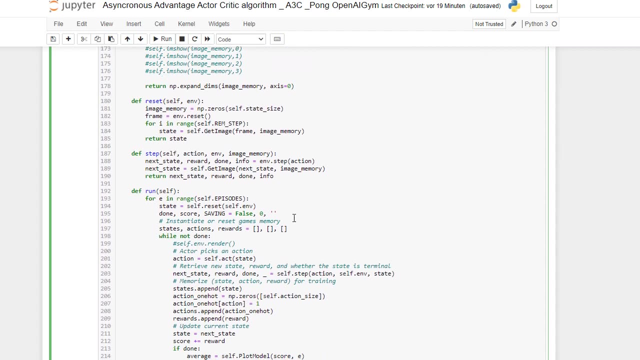 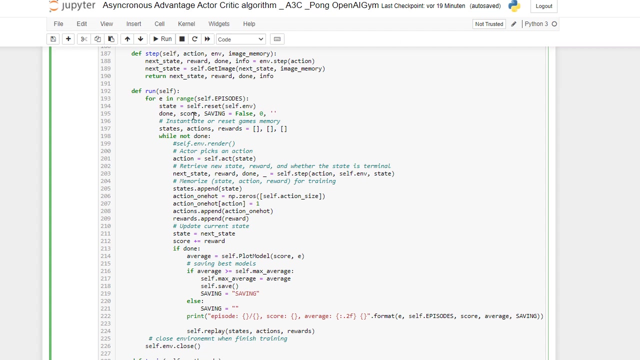 everything you know, the score and steps. we will see afterwards the plotting of the result. The same is here with the get image method, which is going to be used for plotting everything. So the result after the training, Then this run function is important here because this is actually going to be used in the main. 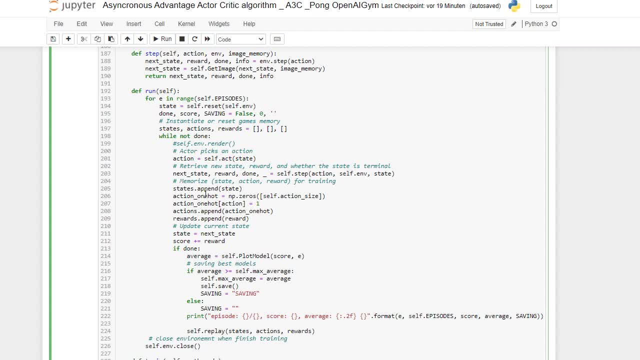 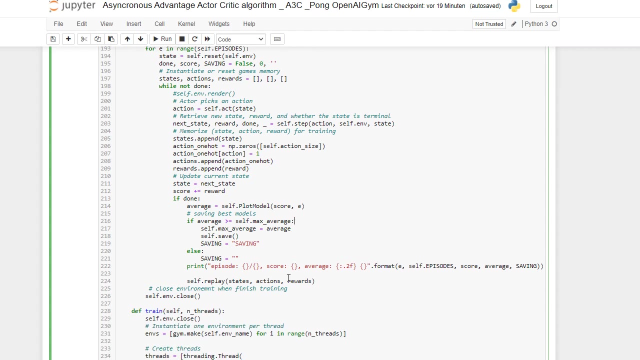 methods afterwards to just do the one hot encoding, to memorize, to retrieve new states, to update current states, to saving best model. So if the model is better than the max average, you can save it actually, And it's going to be trained and plotted everything. 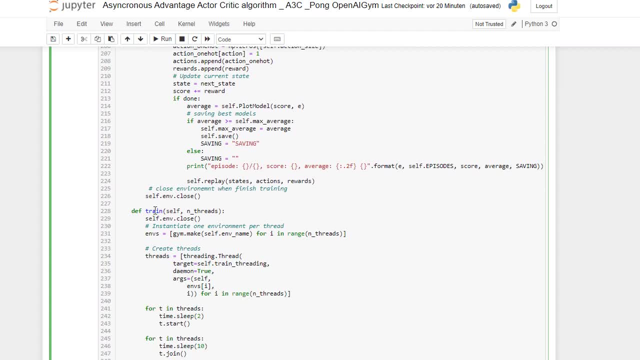 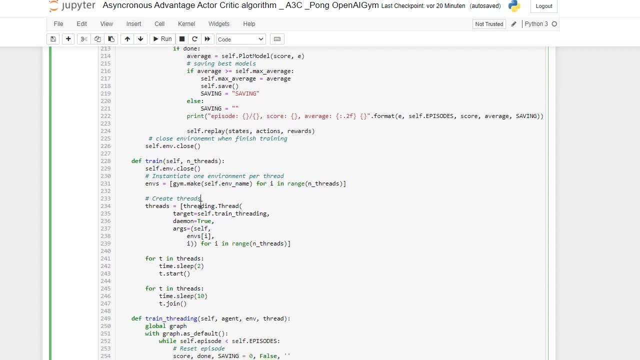 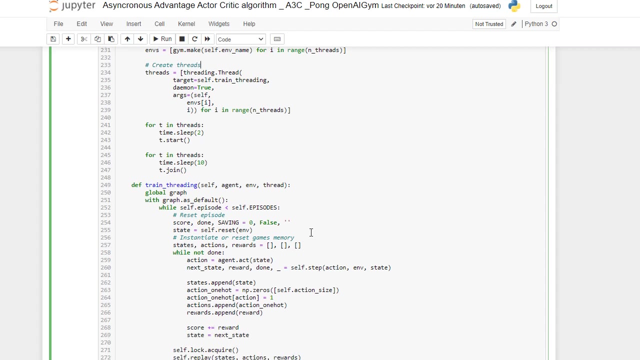 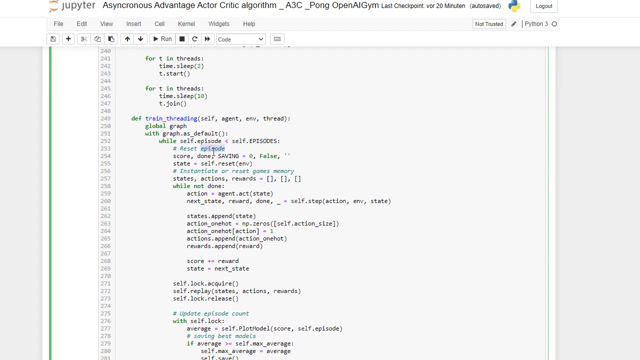 Then this run method is using the train method here to just starting the training to instantly one environment per treat. It's creating the treats itself And afterwards we are also setting up the training treating method to reset the run methods. That's the episodes. 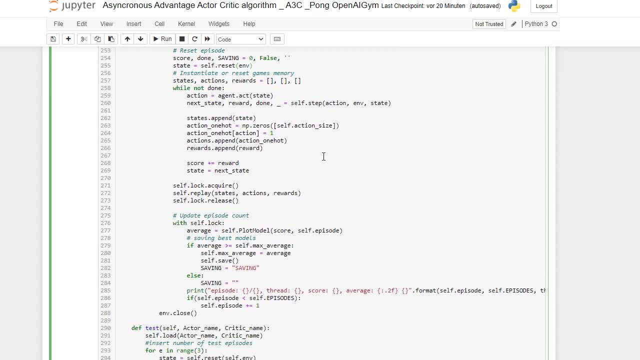 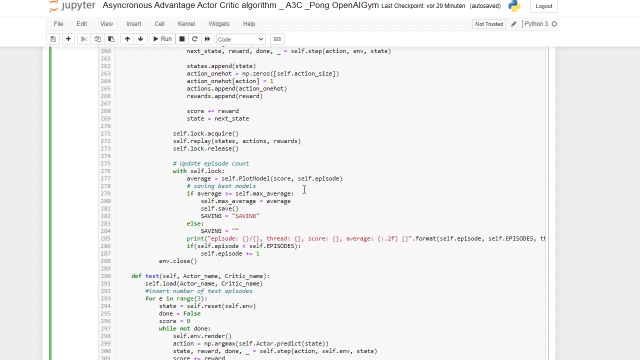 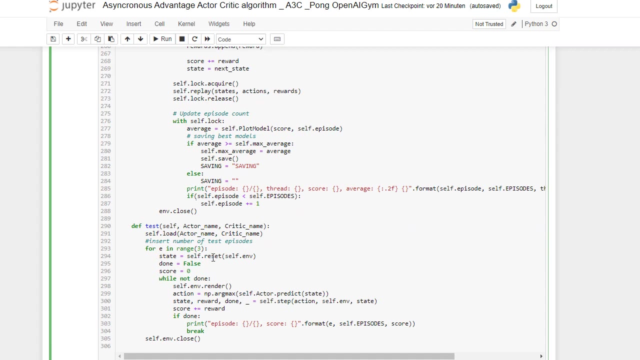 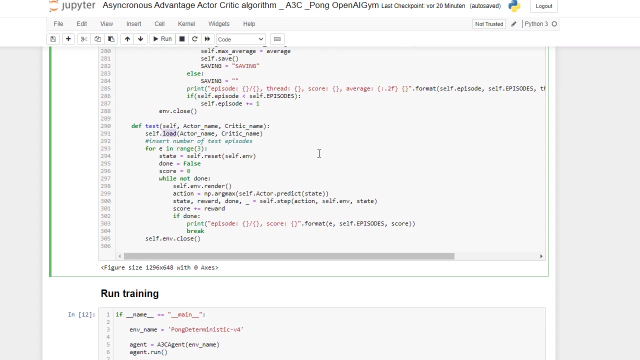 Then we update each episode count, saving the best model again after updating the weights and so on and so on. So then we are plotting everything to just see how the training looks like, to have a little bit more insight due to training. Then the test method is actually going to load the trained model which we saved before. 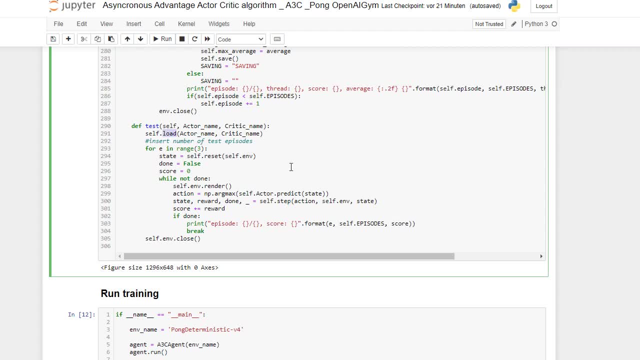 And then the test method is actually going to load the trained model which we saved before To just here. in this case I set up to three because I just want to have three games, that you're not too bored to see how the two guys are playing pong. 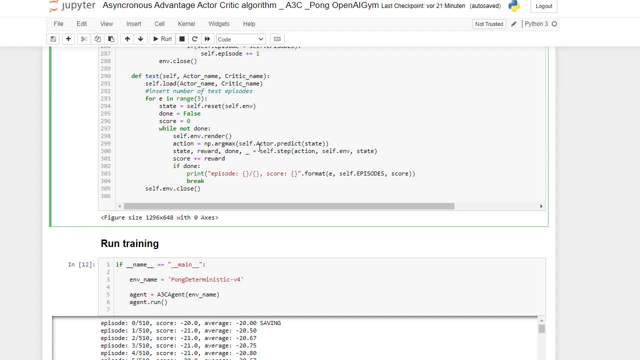 And yeah, you can just see how the predictor, prediction of the actor looks like, because we weren't trained the actor And but and critical as well- but the only the actor is going the model from the actors on only going to be. 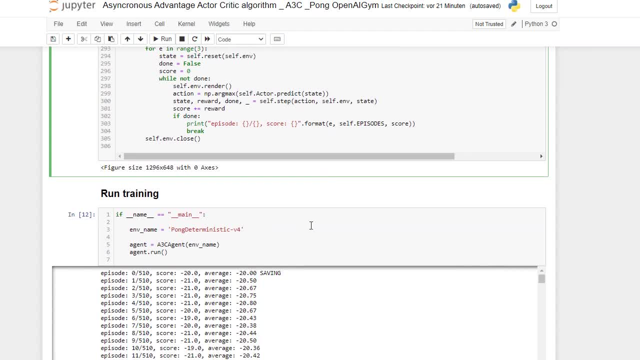 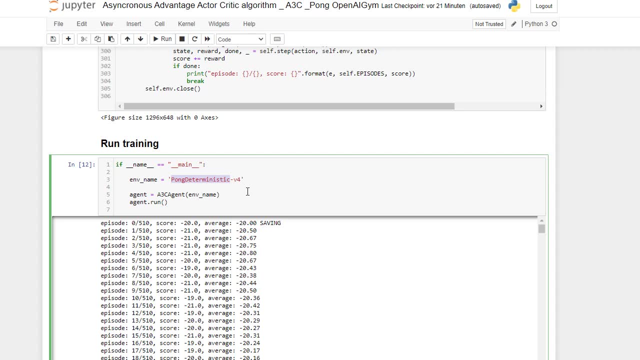 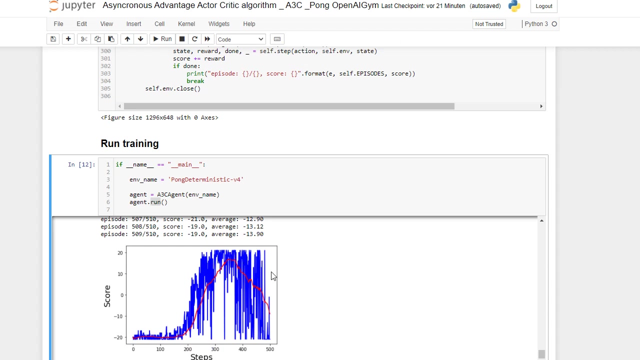 be saved. and then, yes, you can see, here i was using the pong deterministic model because it's going to be faster than the normal pong environment, and i run the method and you can see, after i was calculating 500, you can see that of course the average square is going a little bit down. but 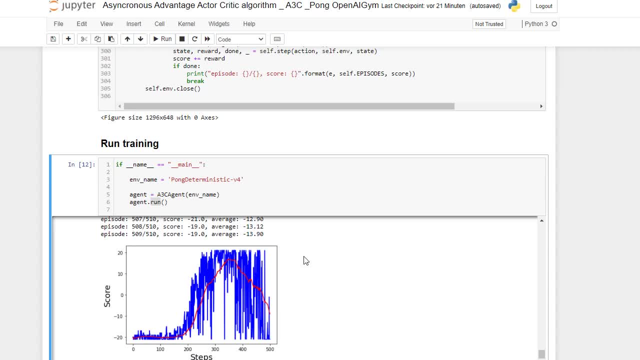 um, after 350 episodes you can see a scoring around about 20, so it's it's actually the goal and you can see that he's really improving after a while, better and better. the red one is the average reward and this is the kind of noisy um reward um over the steps and 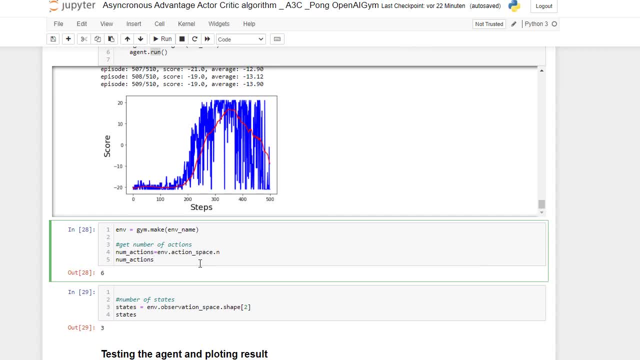 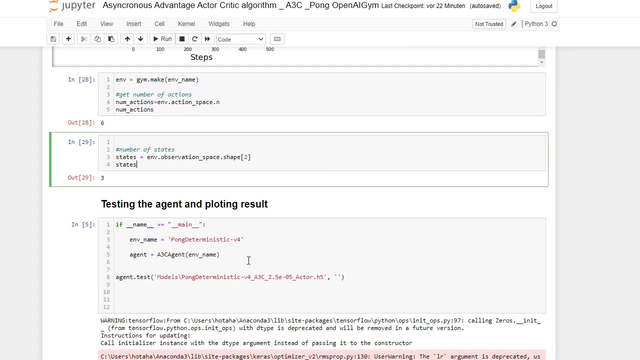 to yeah, and then you can see the number of the action. it's six, you can plot it, the number of states, of course, and um, to just see the result. right, because you're thinking to yourself: why is talking to me so long? i mean, i just want to see the result, i just want to. 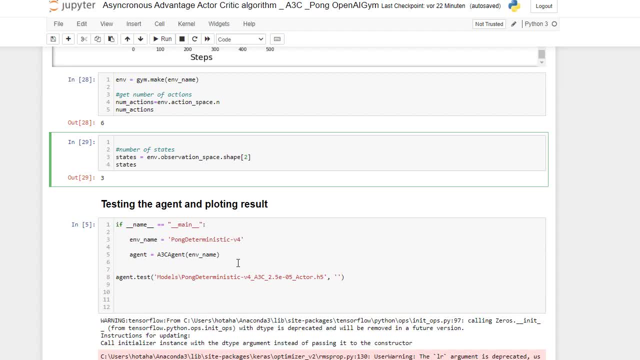 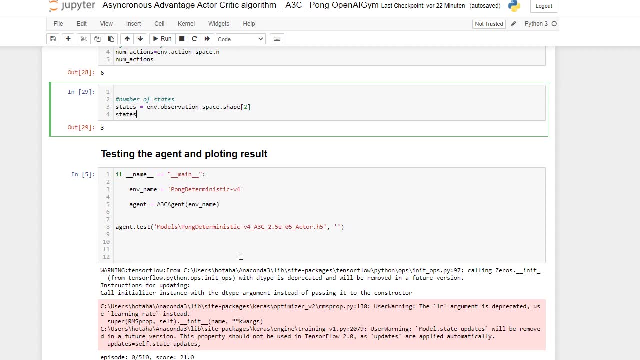 see the performance actually of the f3c agent, why he's improving more than the 83 agent, right? so you can just basically start the test method to just see your saved model how the agent is now performing. so that's why we are going to do this. i'm testing it. 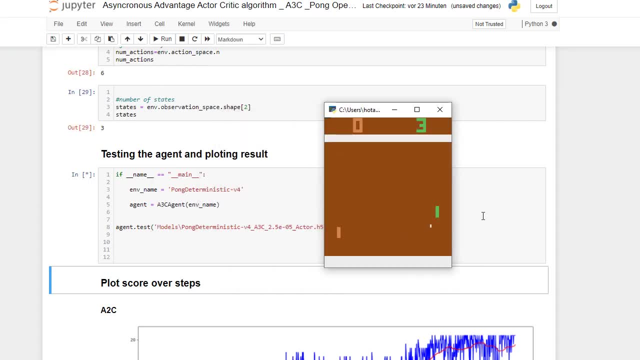 and then you can see that the red one is the trained agent, the green one on the right side and you can see the other guy has no chance anymore. so he's really performing really good. he's really good trained and you can see that he's really fast. 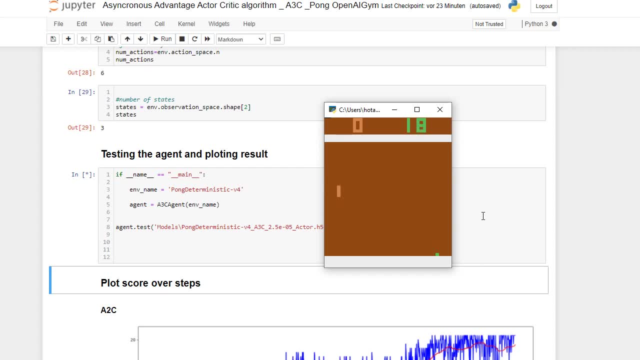 so the red one we can see he's really fast and he's really good at it. so he's a bit chaotic, uh, and a little bit nervous, but he's really playing a good game. so you can see after the first 20 score: so that's the first game he's receiving 24 to 21 score. so he won the first game. 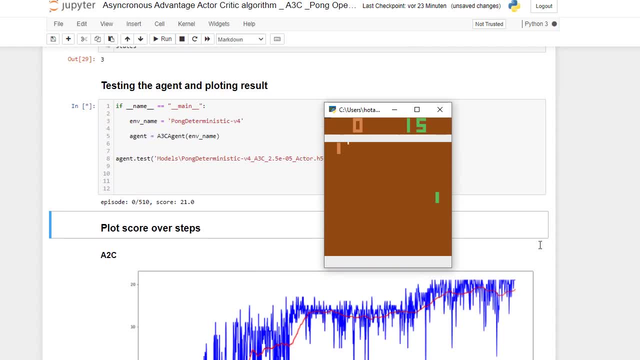 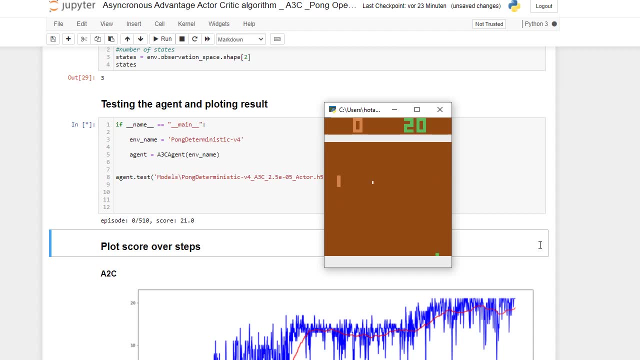 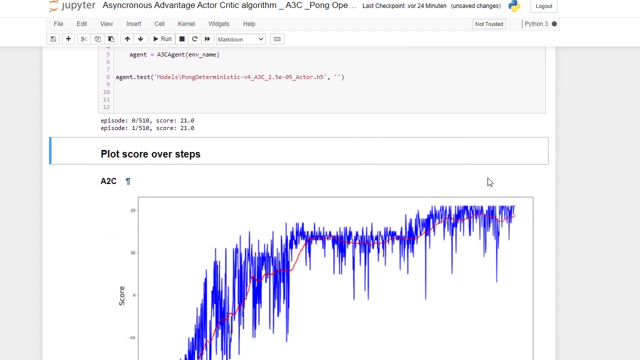 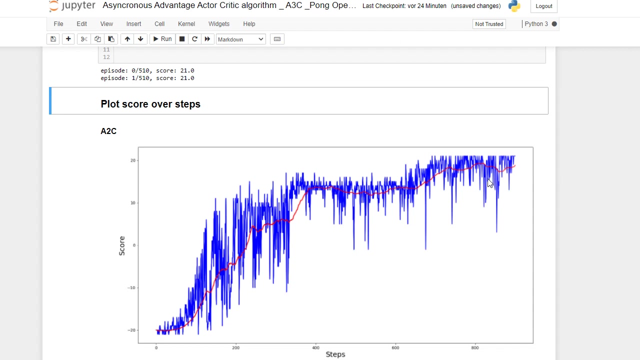 the second game, of course he will also win, so he's even better than the other agent from the environment- Perfect. So he's receiving 21 again. so it's really nice- The model itself performed really good- And to just see the plot of the score or the reward itself over the steps, to just recap.